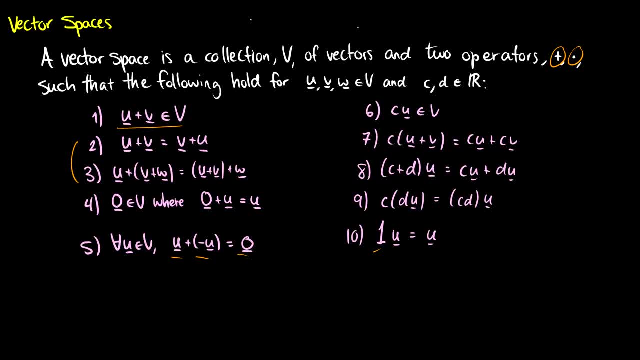 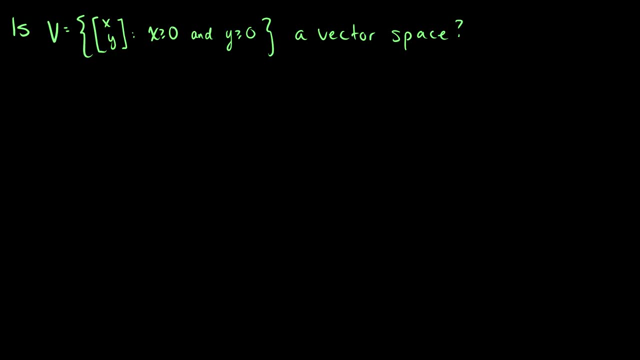 numbers. So let's talk about different things that may or may not be vector spaces. So, for instance, we know the real numbers. this is a good vector space. However, here's a question: Is v, the set of all vectors x, y, where x is greater than zero and y is greater than zero, a vector space? So 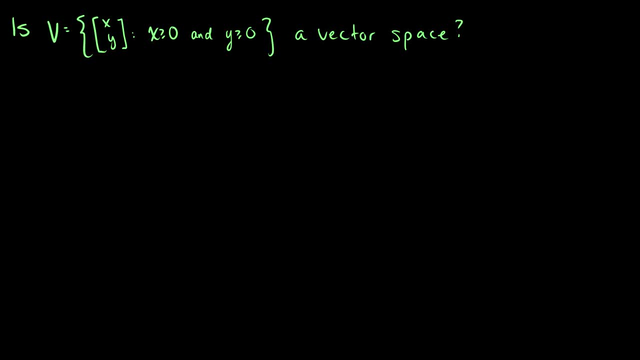 if we take a look, I really don't want to draw r2.. But we're asking: is all this area right here? is this a vector space? So we have to ask ourselves: does it satisfy the axioms? And there's a ton of axioms. 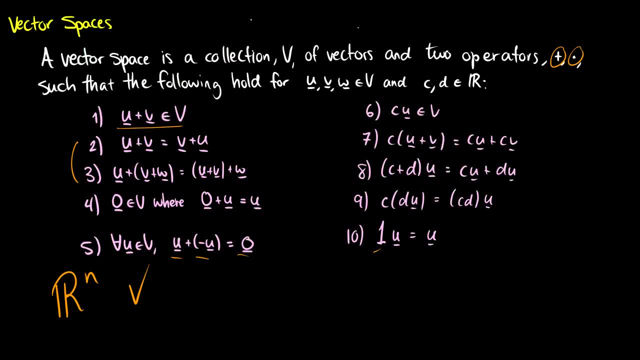 here. So I'm going to circle the two that you should focus on when you're trying to disprove vector spaces. So here's one. Well, let me do that in yellow. So u plus v needs to be in there, And if we multiply by a scalar, it also needs to be in our vector space. And this scalar. 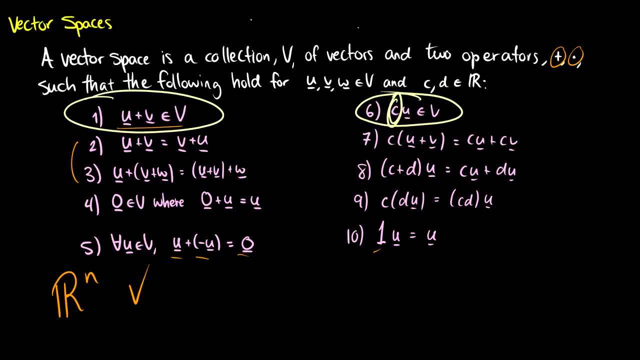 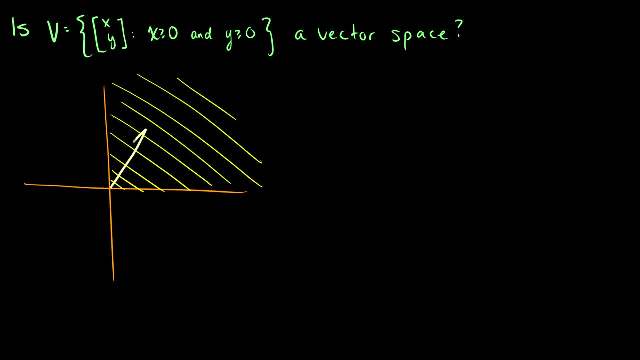 can be any number in the reals, positive or negative. So let's think about this. Okay, So let's say we have a vector like this: It goes out to x, y, It goes to this point. So this is our. 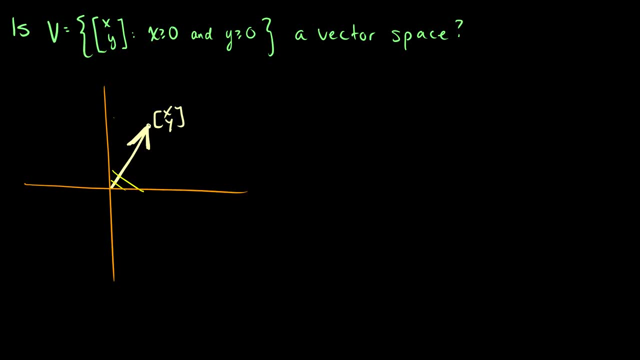 vector x, y. Let me erase these yellow bits Now. is there anything we can think of? So we have u plus v has to be in v. So if we take another vector that's in this space, we can add them together. 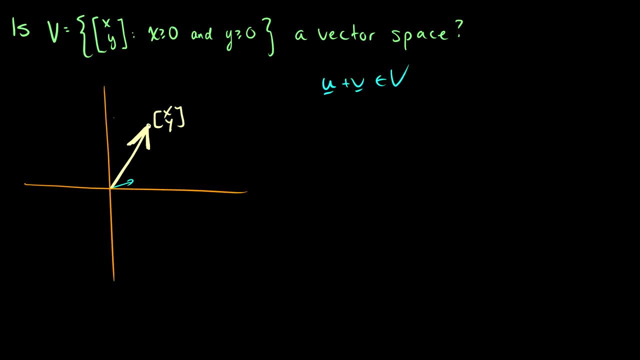 it's going to still be up in this first quadrant here. So that's fine, That's fine. But what if we take a scalar here? So what happens if we scale this by negative 1?? So let's take negative 1 x. 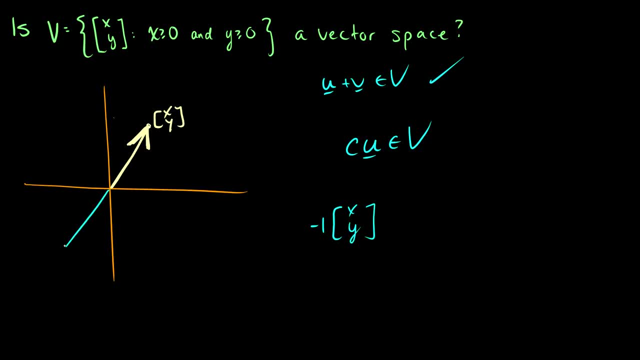 y. Well, what happens then? Well then we end up over here, And this isn't good, because we've exited our vector space. Our vector spaces have to be closed. under addition to multiplication, which means we should never be able to leave this area up here, But if we multiply by negative 1, we can leave our vector space And 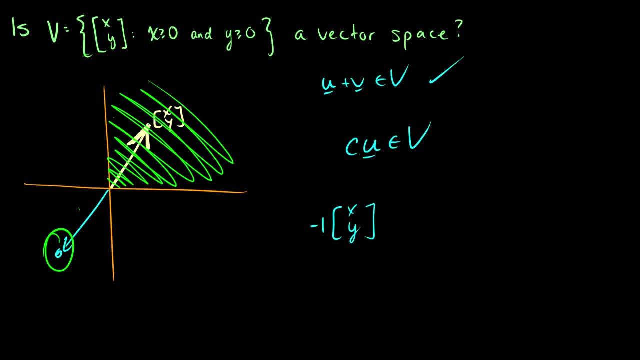 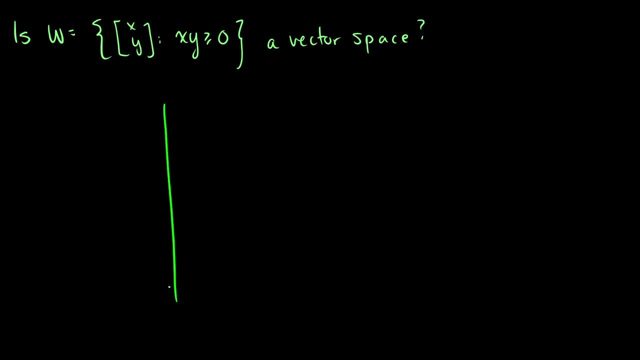 y equals 0.. So if we draw this, this is a little bit different. So we're allowing this space up here, because if we have a positive times a positive, it equals a positive, But we're also allowing this area down here. So a negative times a negative is equal to positive. So this looks. 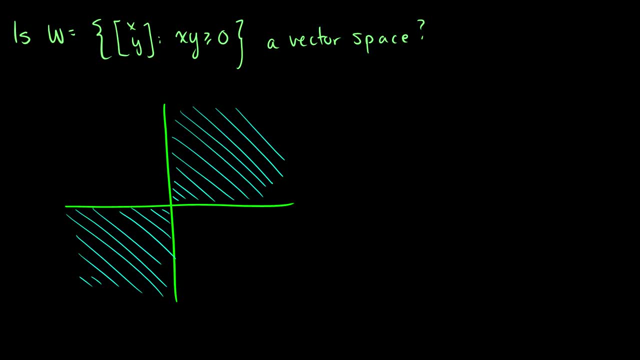 good, right. Okay, well, to disprove this. we want to end up with a vector somewhere in this space, and we can do this by adding or by multiplying. Now what happens if we multiply? What if we take any vector u and multiply it by some scalar c? Well, if it's up here, we're going to end up down. 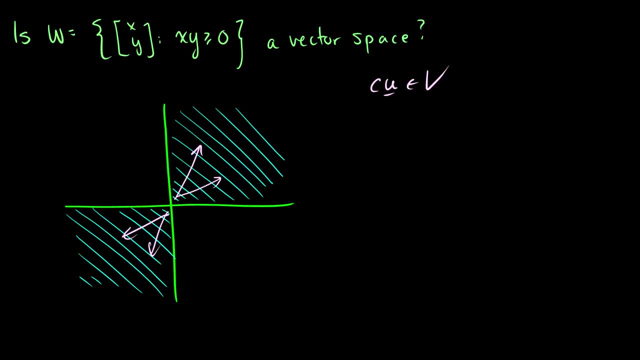 here. If it's down here, we're going to end up up here. So these multiplication tricks aren't going to work for this one. Instead, we should probably find two vectors, when added together, that aren't going to be in our vector space, So we can draw this out and we can draw this out, and we can. 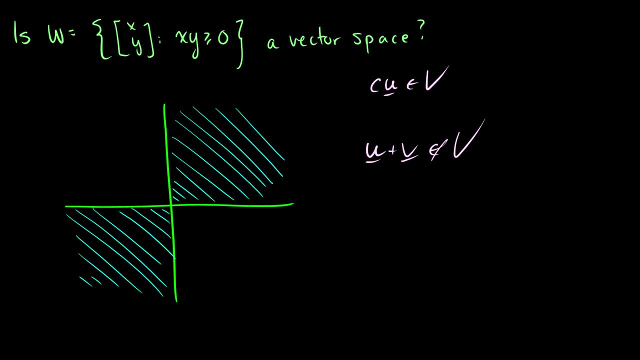 kind of see. So visualizing these things is a pretty good tip, especially at the beginner level. Normally you shouldn't, because things can get abstract really quick. But just for the sake of showing you, let's draw two vectors. that ends up somewhere in this space. Okay, well, we can do one. 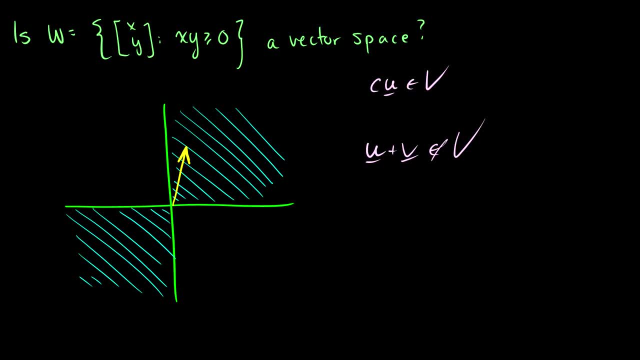 that's pretty straight up, And then we can do one that goes to the left a lot. So when we add these two together- let's do this with brighter yellow- we'd end up somewhere. So what could that look like? We just have to find one pair of vectors that do this. Let's think about 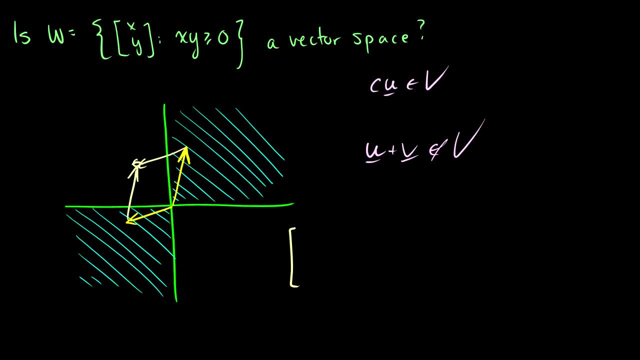 this: You want one to the right and two up, And then we want something like three to the left and one down or something, So we could do minus three and we could do one. Wait, this does not work. This also has to be minus one, So remember. 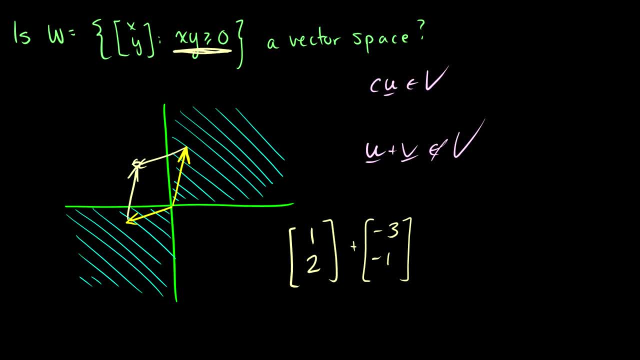 we have to add two vectors to the left, and we can do one. So we can do minus three and we can do one. So we just have that x times y is greater or equal to zero. So when we choose our vectors here, 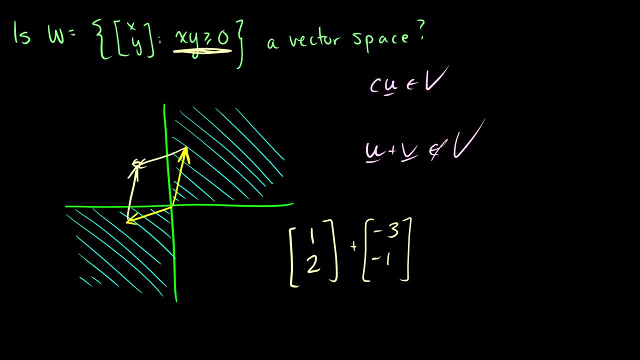 we have to make sure that both of them are in our vector space. So we're good here because one times two is greater than zero. We're good here because negative three times negative one is greater than zero. So this is going to give us negative two and one, And we can see here that our x times y here. 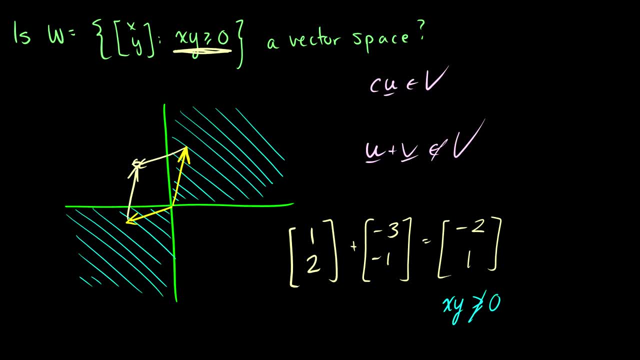 is definitely not greater than zero. Therefore, this is also not a vector space. So you can see we're pretty limited to what our vector spaces are. If we're working in the plane R2, it's probably going to have to be most of R2.. Now, of course, there are some exceptions here. 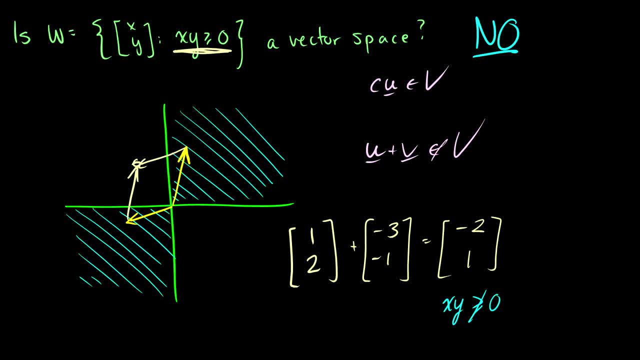 We'll talk about those eventually. But drawing diagrams like this and visualizing, especially when you're first starting, is a great way to figure out what a vector space is. So you have to play with numbers, You have to play with these axioms and see which ones are violated Again. 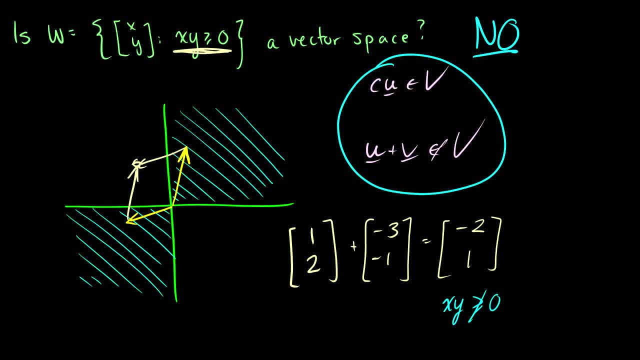 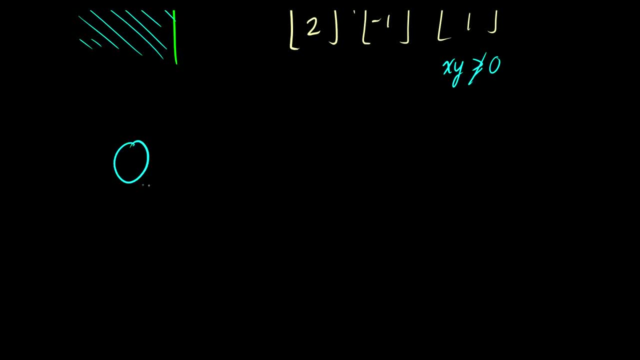 these two are great. Let's check to see if they're violating. Another one to check- that is usually on trick questions- is: is the zero vector in your vector space? Because sometimes you may be given vector spaces where you can't get the zero vector And those are not vector spaces. So you must check for those. 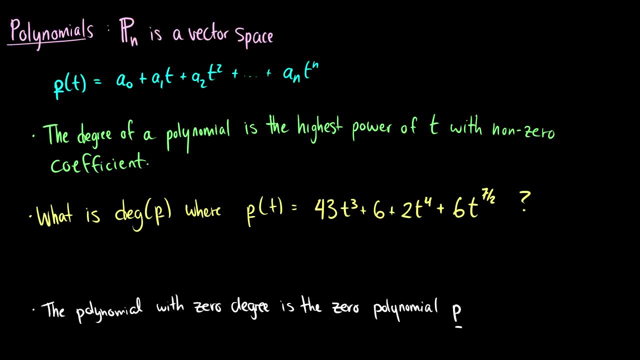 Okay, here's one that might surprise you. Polynomials are a vector space. So, for instance, we can write a polynomial as a0.. a0 plus a1 times t plus a2 times t squared, And this just goes up to some t, to the n. 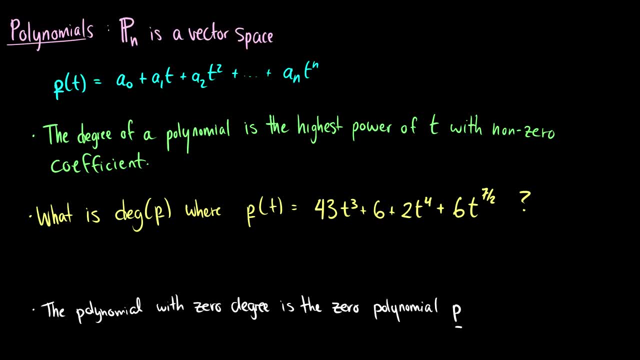 So this might be a new notation for polynomials, if you've never actually looked at polynomials before. But these are just constants, these a0s and a1s, So you can kind of see they look like vectors. So we need some notation here. The degree of a polynomial is going to be the. 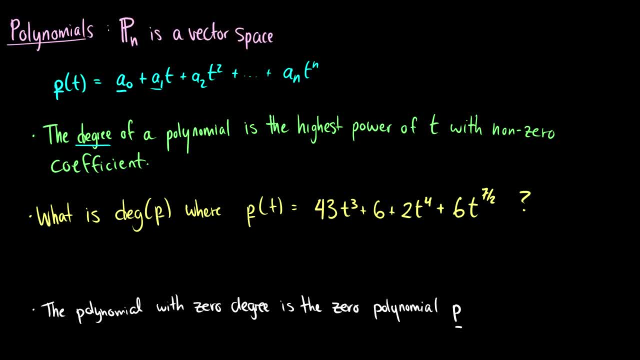 highest power of t that is non-zero. So in this first example, assuming that a is not equal to zero, then the degree of this polynomial would be n. So that's n degree. So, for an example, what is the degree of p where we have the polynomial 43t cubed plus 6? 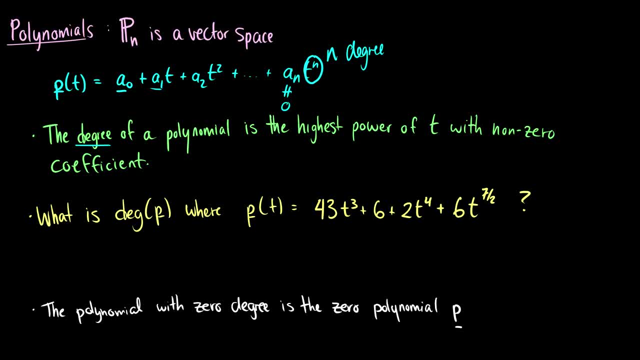 plus 2t to the 4, plus 6t to the 7, halves. Well, this is the same thing as 3.5,. our highest power is t to the 4.. So the degree of of the vector P or the polynomial P is going to be 4.. The polynomial with the 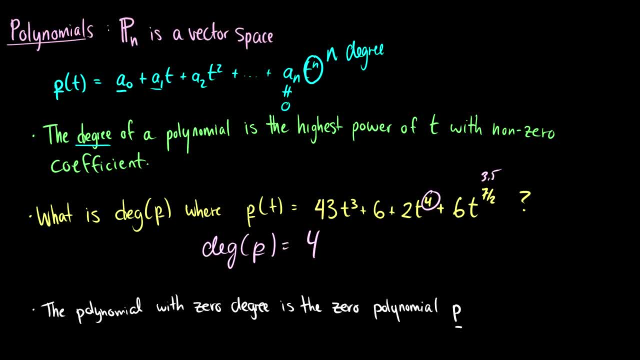 zero degree is the zero polynomial, so this is usually just again written as a zero. So this is the nice thing about when talking about vector spaces is we know what the zero means. This could be the zero for anything, so we just use the. 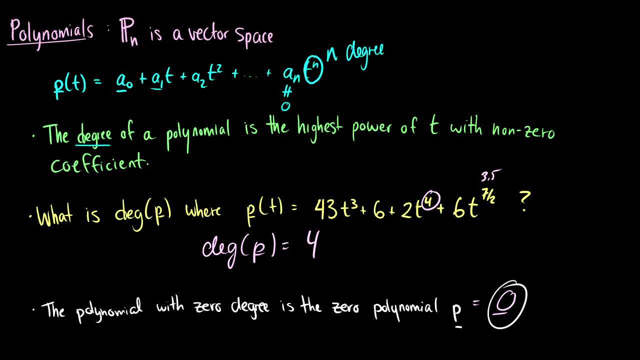 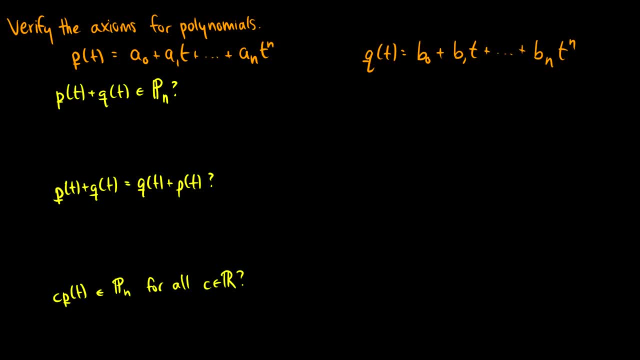 same symbol here to denote that. So the zero with the bar under it. that's good, In fact, for polynomials. sometimes it doesn't even have the bar. Okay, so let's verify the axioms for polynomials, because I kind of just told you that. 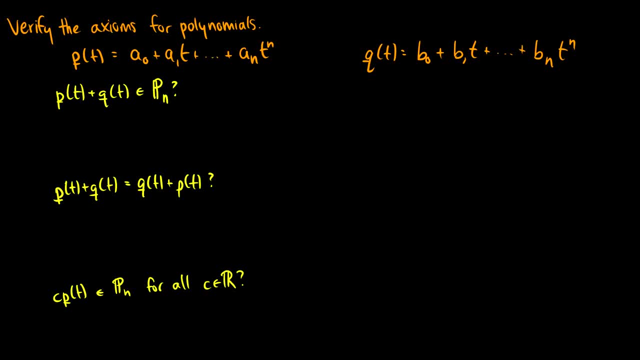 it's a vector space, but you might not believe me, so let's prove it. First of all, if two vectors or two polynomials are in the space independently, then there's some has to be in the space as well. So I'm going to write this as a vector space and I'm going to write this as a 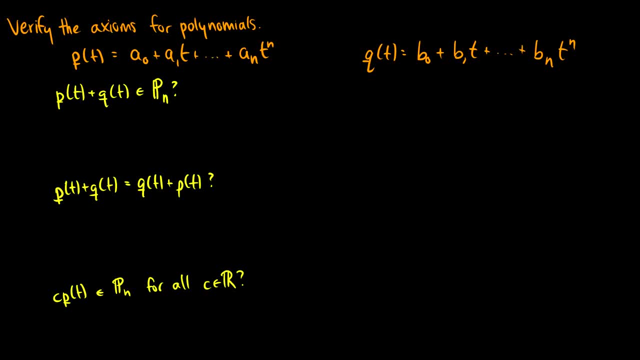 vector space and I've listed P and Q and we can add these together. So, for instance, Pt is going to be a0 plus a1t all the way up to ant, to the n, and then we're going to add our vector Qt. This is going to be b0 plus b1t all the way up. 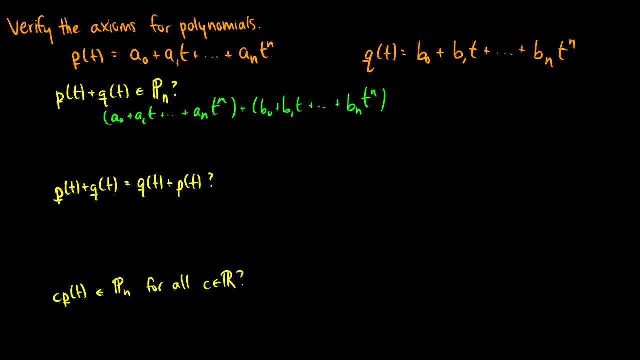 to bn, t to the n I should mention these are the same degree, but they don't have to be, because these are polynomials. So we could add a four degree polynomial with a seven degree polynomial and their end result would be the seventh degree. 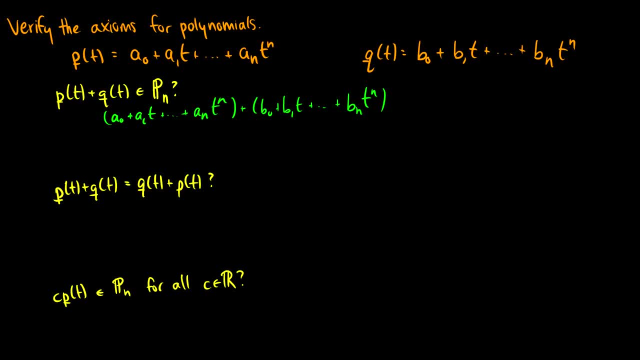 polynomial, You do have to make sure that if you're working in seven degree polynomials, you are in P. This is P specifically, so this has to be less than or equal to that n. Okay, so now what we can do is we can group things up, So 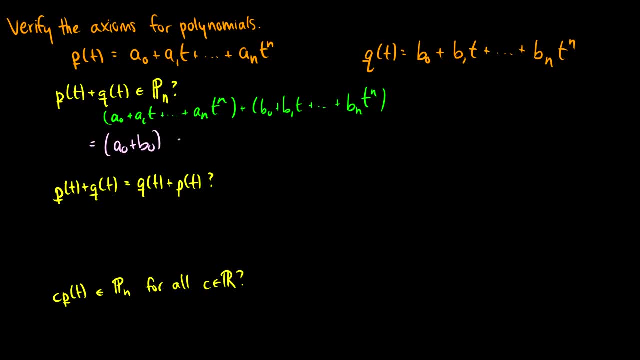 we can take a0 plus b0, then we can add a0 plus b0.. a1 plus b1 times t. This will go all the way up to an plus bn times t to the n. So this is in our space. This is good, All of these are good. Therefore, this axiom, 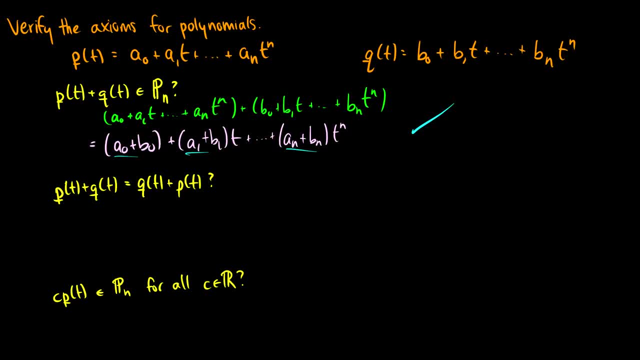 is satisfied. What about if we have polynomial P plus Q? This is equal to Q plus P. Well, we already have this first part here, so I'm just going to take this and we'll write it down. and we know that we can switch the values of this right. We know that we can write this as b0 plus. 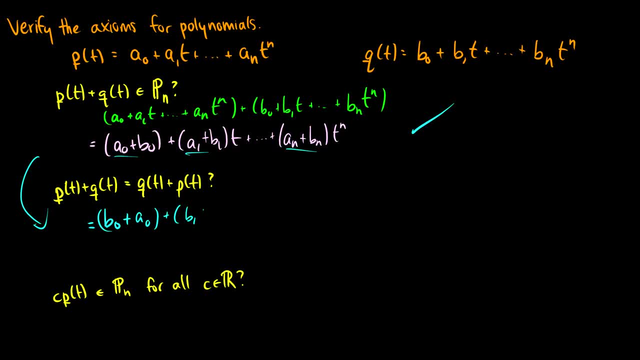 a0, because these are just real numbers. We've already worked with these. So this is b1 plus a1, t all the way up to bn, plus an times t to the n. Then we can separate these again, So we can expand, and then we would end up with b0 plus b1. 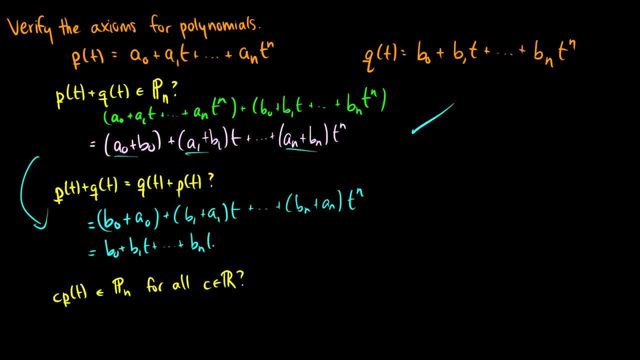 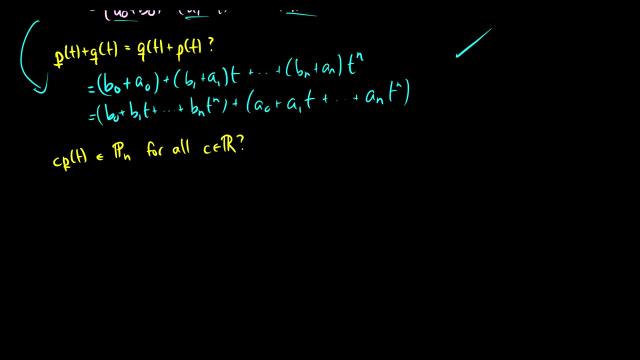 t plus all the way up to bn, t to the n. Then we could add our a0 plus 1 t all the way up to a n t to the n. So the second axiom is good too. What about this third one? If we take a constant and we multiply it for all c, well, first of all we have a 0 plus a 1 t. 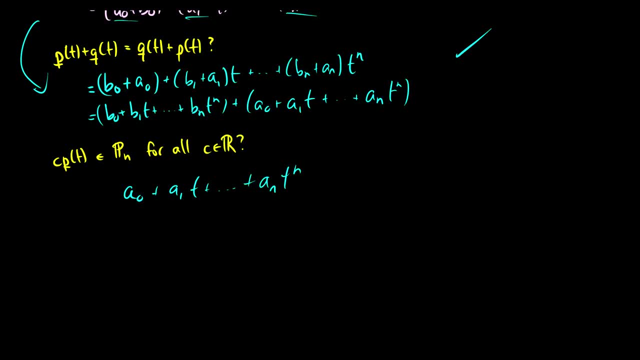 all the way up to a, n, t to the n, and let's multiply that by some constant c. Well then we just end up with c times a, 0 plus c times a, 1 times t, all the way up to c, a n times t to the power of n, and we're good. So these were three of the axioms. With these. 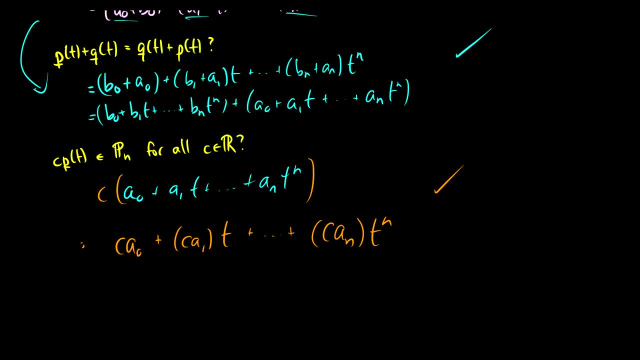 three axioms. you can prove everything else pretty straightforwardly. So if you want the practice, you can prove the remaining seven, but you really don't have to, because you should see things follow from this pretty simply. For practice, though, I'd suggest doing it. But that is it for vector spaces. Next video is subspaces. 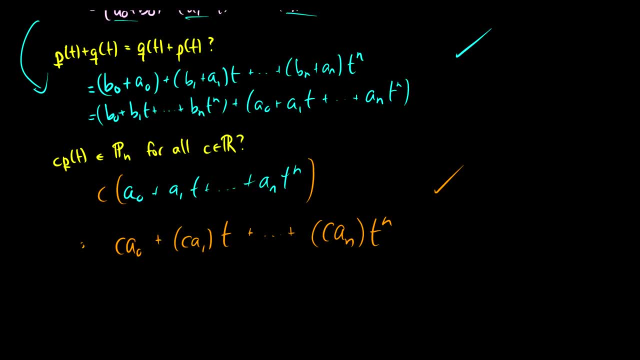 and I'll see you guys. then, If you have any questions, please leave them in the comments below and I'll answer them as quickly as I can.